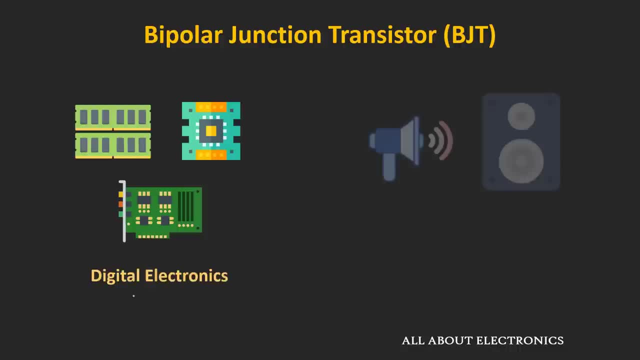 or it can be used as an amplifier in the analog electronics. So nowadays the field effect transistors are widely used in the electronic industry, But still the BJTs are extensively used And anyone who is interested in electronics should have some basic knowledge of this BJT. 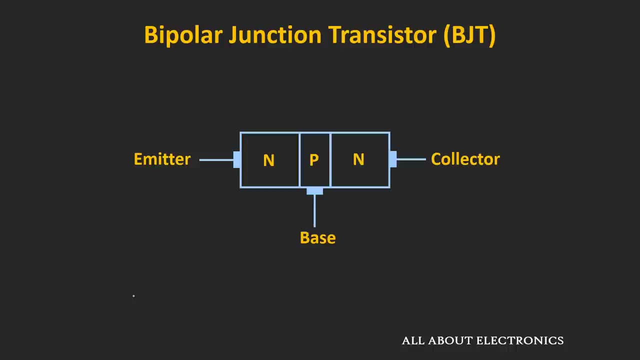 So in this bipolar junction transistor there are three doped regions: the emitter, the base and the collector- And, based on the doping of these three regions, it is known as either the NPN or the PNP transistor. So in case of the NPN transistor, there are 3 doped regions. So this is the three doped. 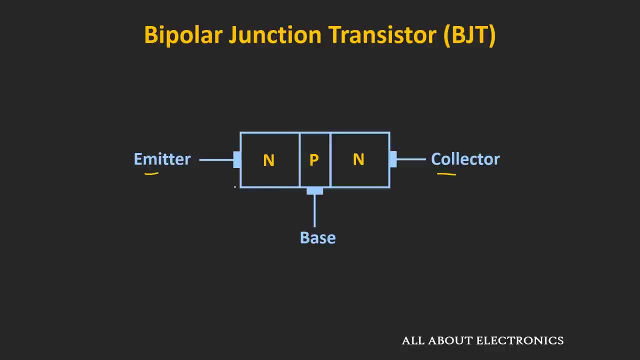 transistor, both emitter and the collector are doped with the n-type impurity and the base is doped with the p-type impurity. On the other end, in the PNP transistor, the base is doped with the n-type impurity and the emitter and the collectors are doped with. 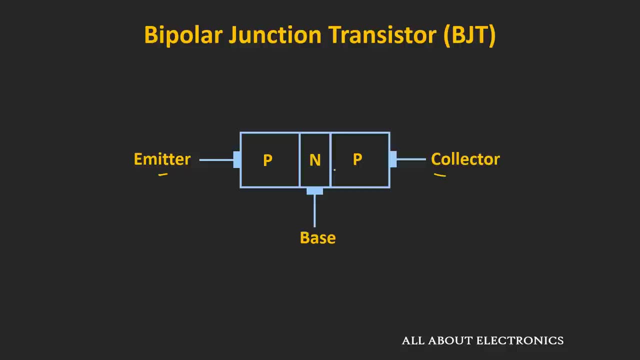 the p-type impurity, And here the term bipolar indicates that both electrons and holes contribute in the flow of current. Now, if you look inside this BJT, then there are two PN junctions: One is between the emitter and the base, And second is between the base and the collector. 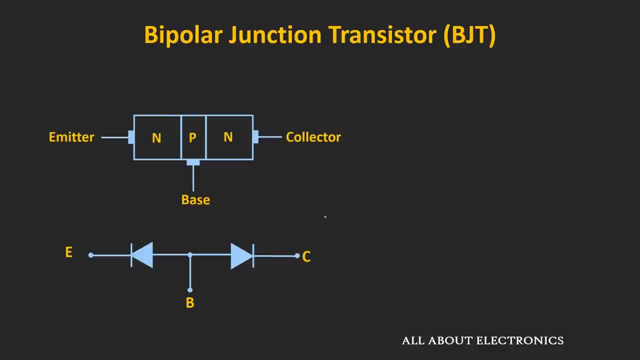 And it appears as if the two back-to-back diodes are connected in the series. But actually it won't behave like that, Because when we connect two back-to-back diodes, then we are assuming that there is no interaction between the two diodes. 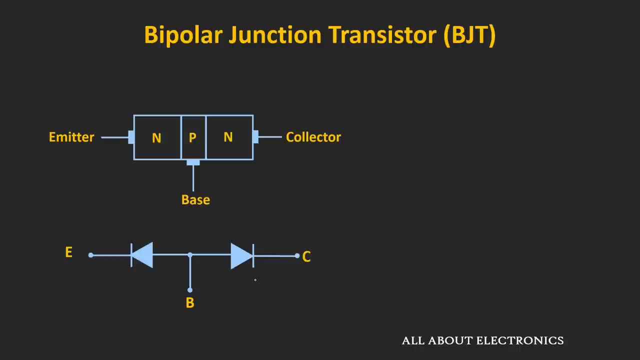 That means these two diodes are operating independently. But in case of the BJT, actually there is a n-type impurity. There is an interaction between the two regions. So if we connect the two back-to-back diodes like this, then it won't behave like a BJT. 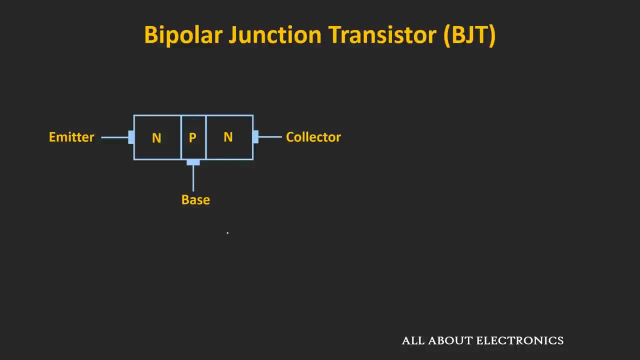 Now, if we talk about the internal construction of the BJT, then the emitter is heavily doped and the function of the emitter is to supply the electron And in fact that is why it is known as the emitter. Then if we talk about the base, then it is lightly doped and the doping concentration 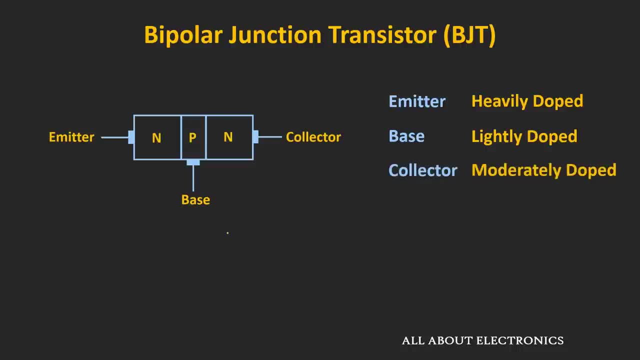 of the collector is between the emitter and the base. That means the collector is the moderately doped. And if we talk about the width of these three regions, then the base region is much narrower compared to the two regions. So in terms of the width, the collector region is wider than the other two regions. 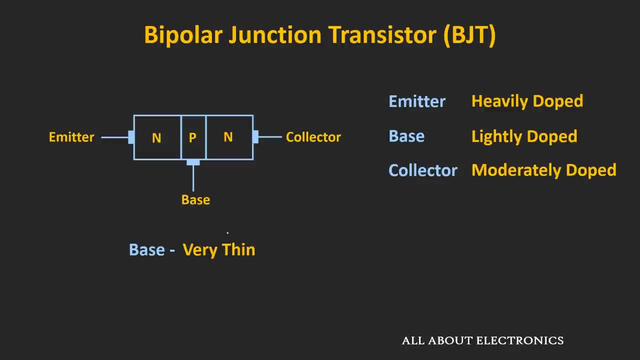 Because the job of the collector region is to collect the electrons which is supplied by the emitter And in fact, that is why it is known as the collector. Now, depending on the biasing, the BJT can be operated in three ways. 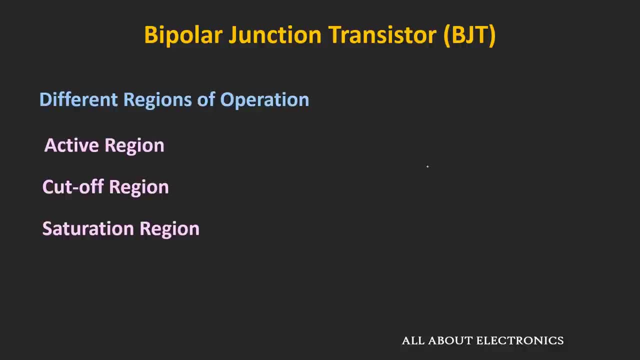 The first is the collector, The second is the emitter, The third is the collector And the last one is the emitter. So we have three regions: The active region, the cut-off region and the saturation region. So in case of the active region of operation, the emitter-base junction is forward biased. 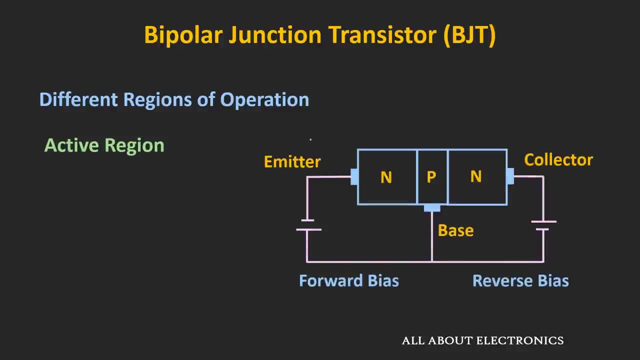 and the base-collector junction is reversed, biased. So let's say the voltage at the emitter is Ve, the voltage at the base is Vb and the voltage at the collector is Vc. Then to forward bias this base-emitter junction, the voltage of base should be greater than 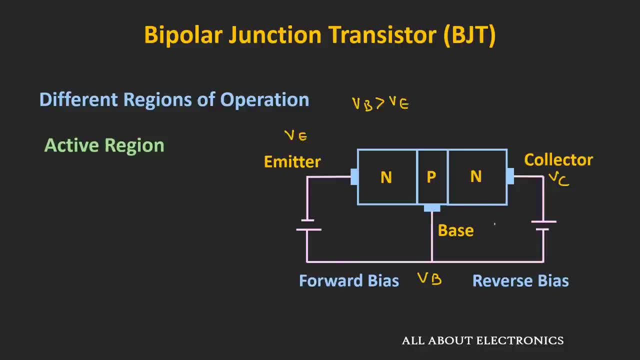 emitter And similarly, to reverse bias this emitter, the collector should be reversed, biased. To reverse bias, this collector-base junction, the voltage at the collector should be greater than base. That means to operate the BJT in the active region. we can say that the collector voltage 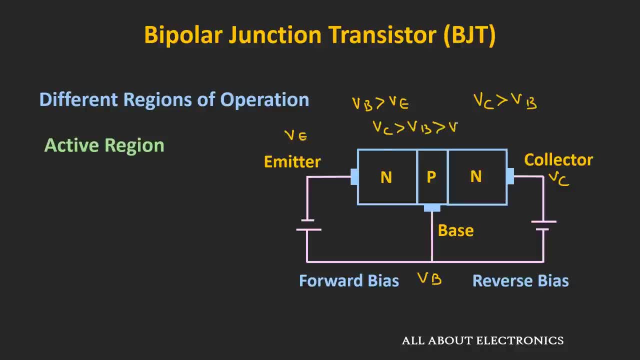 should be greater than base voltage and the base voltage should be greater than emitter voltage. So once this condition is satisfied, then the BJT will operate in the active region. Similarly in the cut-off region, both base-emitter junction and the base-collector junctions. 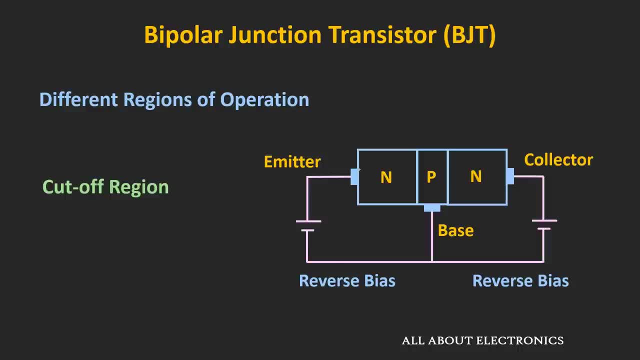 are reverse biased. So to operate the BJT in this region, the emitter voltage should be greater than base voltage and at the same time the collector voltage should also be greater than base voltage. Similarly, in case of the saturation region of operation, both base-emitter and the base-collector 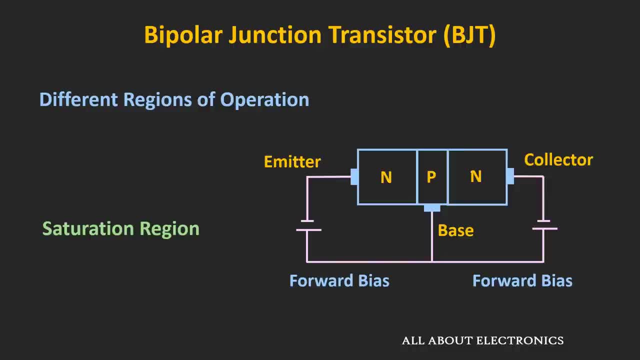 junction of the BJTs are forward biased. That means in this region of operation the base voltage, VB, is greater than emitter voltage and at the same time This is true Because base voltage is also greater than collector voltage. So these are the three regions of operation in case of the BJT. 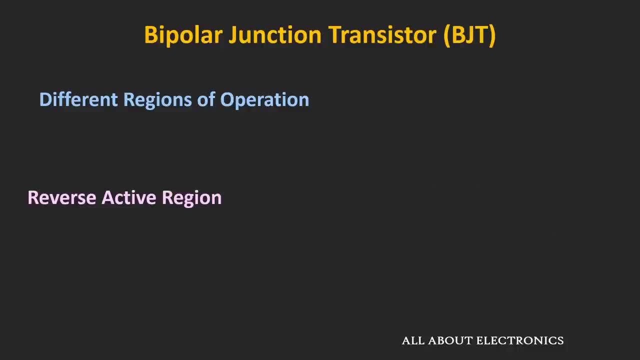 Apart from that, there is one more region of operation, which is known as the reverse active region of operation. So in this region of operation, instead of base-emitter junction, here the base-collector junction is forward biased and the base-emitter junction is reverse biased. 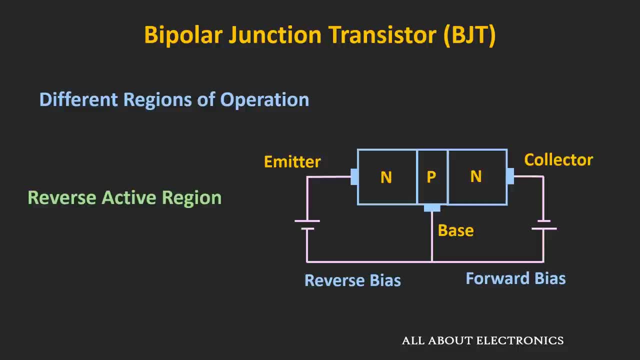 But in this region of operation the gain provided by the BJT is very less. Due to that, this region of operation is usually avoided. Similarly, if we talk about the PNP transistor, then in case of the active region of operation, 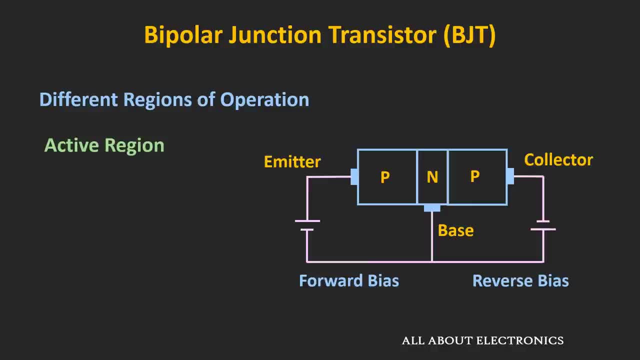 this base-emitter junction is forward biased and the collector-base junction is reverse biased, But in this case now the emitter voltage is greater than the base voltage and similarly the base voltage is greater than collector voltage. So we can say that in case of the PNP transistor to operate it in the active region, then the 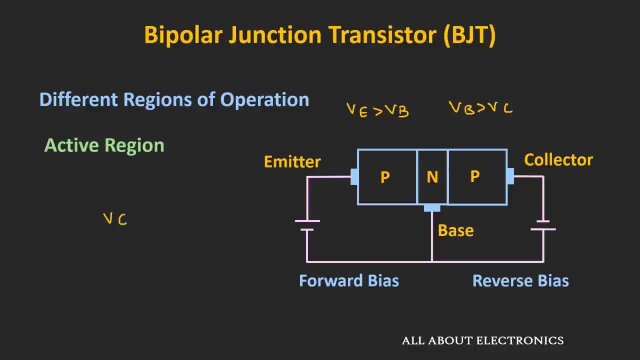 base-emitter junction is forward biased and the collector-base junction is reverse biased. But in this case now the emitter voltage is greater than the base voltage and similarly the base-emitter junction is forward biased and the collector-base junction is reverse biased. 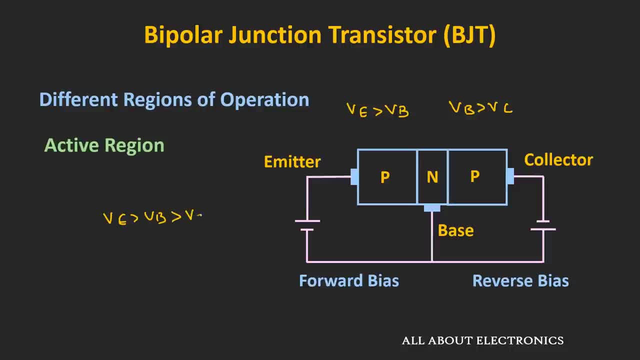 So in this case, in the active region, the emitter voltage should be greater than the base voltage and the base voltage should be greater than the collector voltage. And similarly this PNP transistor can also be used in the different regions. So whenever the BJT is used for the amplification, then it is used in this active region and 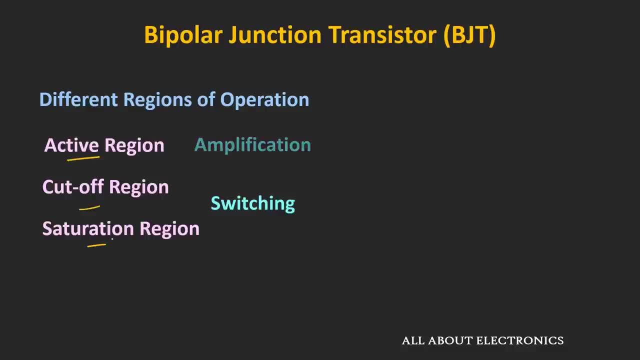 whenever it is used as a switch, then it is used in the saturation and the cut-off region, And in the upcoming videos we will see in detail about these different regions of operation. Now, if we talk about the symbol, then this is the symbol of the NPN transistor. 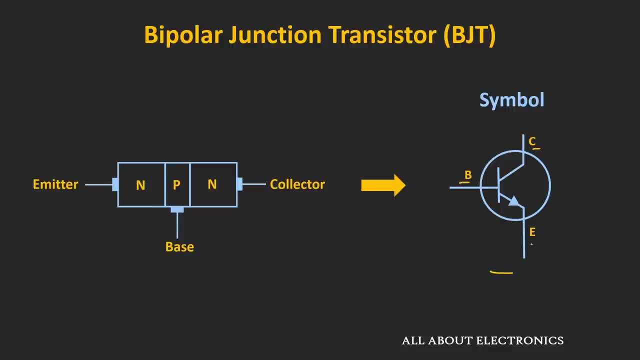 So these three terminals are the base, collector and the emitter, And here this arrow indicates the direction of the current during the active region of operation. So in case of the NPN transistor, the current will flow from the base towards the emitter. 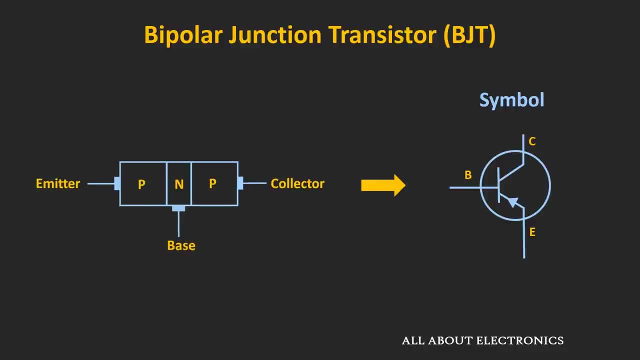 On the other hand, if you see the symbol of the PNP transistor, then it is similar to the NPN transistor, But here the direction of the current is different. So in this case the current will flow from the base towards the emitter. 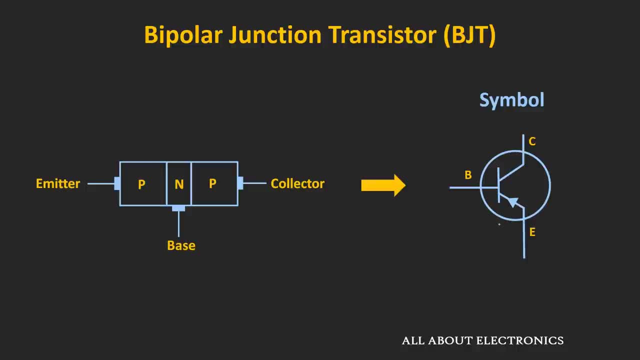 And the direction of the arrow will get reversed. So now the current will flow from the emitter towards the base region. Now, as I said, when the BJT is used for the amplification of the signal, then it is operated in the active region. 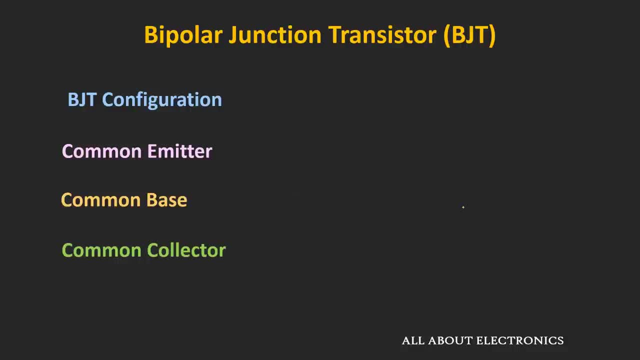 And there are different ways to configure it. So in case of the common emitter configuration, the emitter terminal is common between the input and the output. That means in this configuration the input signal is applied between the base and the emitter And the output is measured between the collector and the emitter terminal. 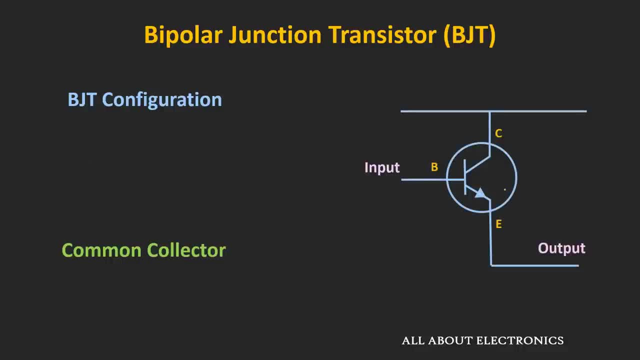 Similarly, in case of the common collector configuration, the collector terminal is common between the input and the output side, And likewise in the common base configuration, the base terminal is common between the input and the output side. So each configuration has its own advantage and disadvantage. 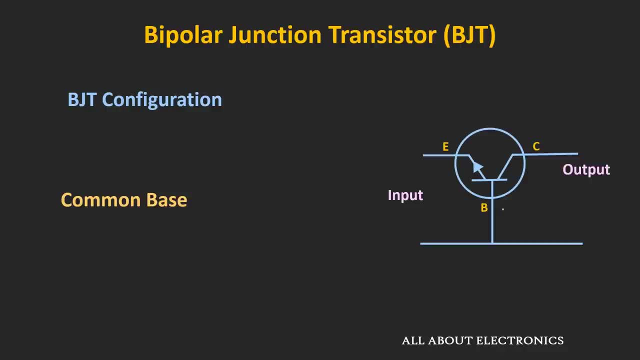 And we will see all these configurations in detail in the upcoming videos. But in short, For the instrument and the application, the BJT can be configured in any of these 3 configurations. Alright, so now let's understand the working of the BJT whenever it is operated in the 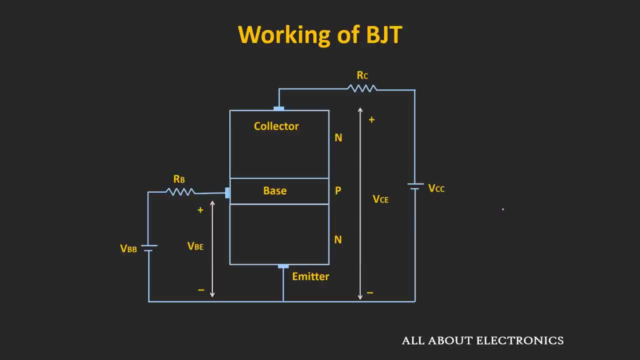 active region, And here we will take the example of the NPN transistor. Now, before we understand the working, let me just clear the notation which is used for the supply voltages. So, as you can see over here, for the base and the collector supplies double subscription. 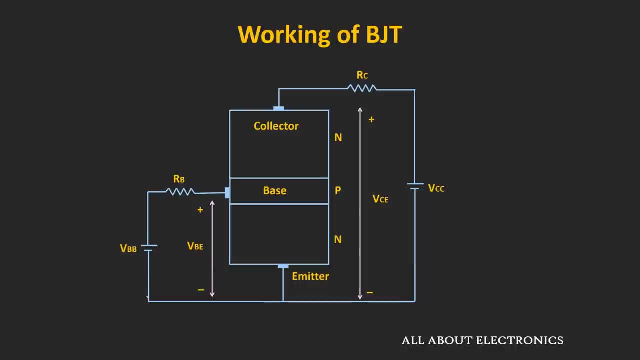 is used. That means Here: this VBB is the source voltage for the base And the VCC is the source voltage which is connected to the collector terminal. And this voltage, VBE, defines the difference between the voltage at the base and the emitter. 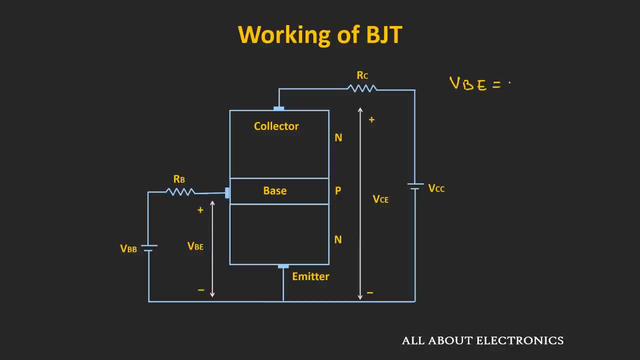 terminal. So this voltage VBE can be defined as voltage VB minus VE. So if the voltage at the base terminal is, let's say, VB and the voltage at the emitter terminal is VE, then the voltage VBE can be defined as voltage VB minus VE. So if the voltage at the base terminal is, let's say, VB and the voltage at the emitter terminal is VE, then the voltage VBE can be defined as voltage VB minus VE. So if the voltage at the base terminal is, let's say, VB and the voltage at the emitter terminal, 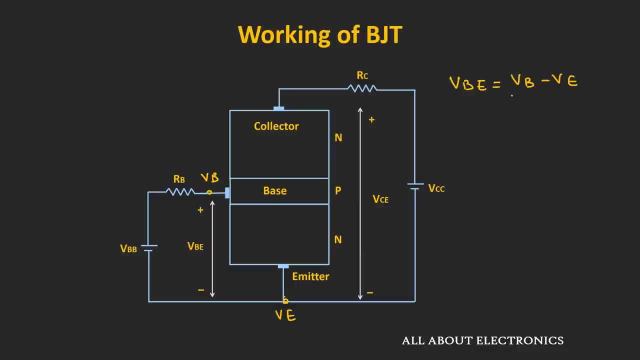 is VE, then the voltage VBE can be defined as voltage VB minus VE, And here this voltage VB and VE are measured with respect to the ground terminal. Similarly, this voltage VCE can be defined as the collector voltage VCE minus VE. 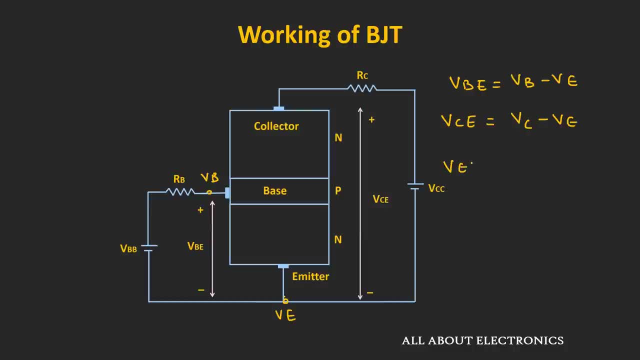 So instead of VBE, if we write voltage VEB, then it can be written as voltage VE minus VB And this voltage will be negative of the VBE. So throughout our discussion on the BJT we will use this notation. 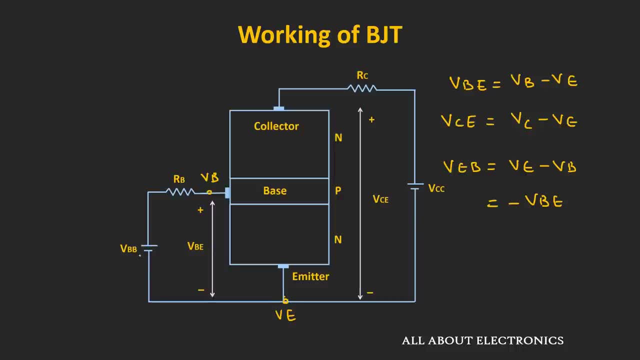 So here this base voltage and the collector voltage is applied in such a way that the base emitter junction will get forward, biased, and the base collector junction will get reversed, biased. That means over here the BJT is biased in such a way that this voltage VBE is positive. 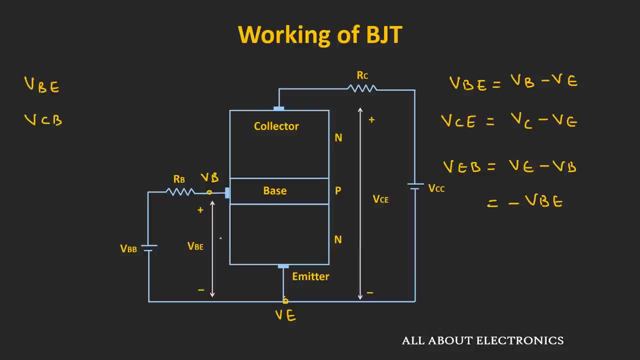 and this voltage VCB is also positive. Now, if you notice over here, this is the PN junction. So whenever this PN junction is forward biased, Then the typical forward voltage drop across this diode is in the range of 0.6 to 0.7 V. 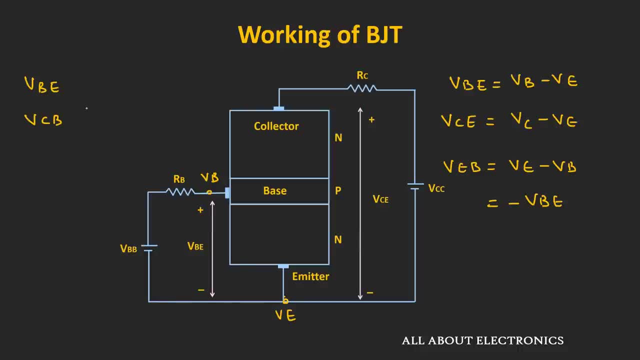 That means whenever we forward bias this base emitter junction, then the typical voltage drop between this base and the emitter junction will be roughly around 0.7 V. Now, once we apply these biasing voltages, then the electrons from the emitter will be. 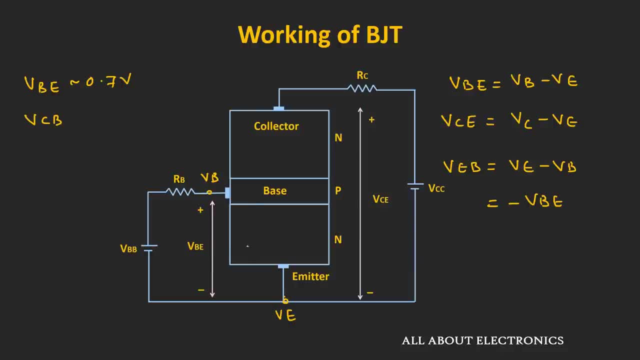 pushed towards the base terminal Because, as I said earlier, the emitter is the heavily doped. That means the emitter has the large number of electrons as the base terminal. So the base emitter is the heavily doped And the electrons are the majority carriers. 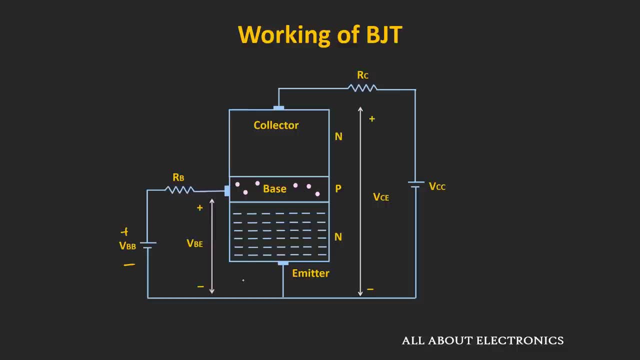 And once we apply this biasing voltage, then this negative voltage will push the electrons towards the base region. So, due to that, the electrons will start moving towards the base region. Now, once the electrons enter this base region, then there are two paths for them. 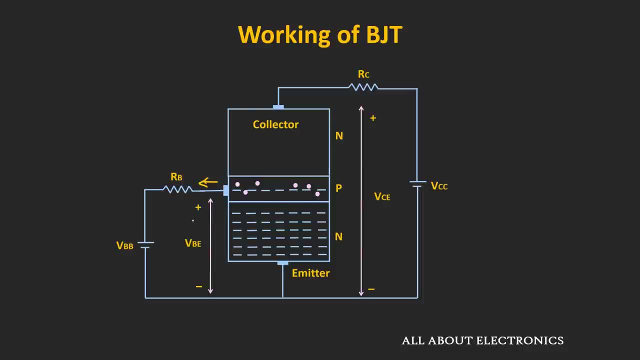 One is they can flow towards the positive terminal on the left And the second is they can flow into the collector region. But most of the electrons will enter into the collector region Because if you see over here, the base is lightly doped. 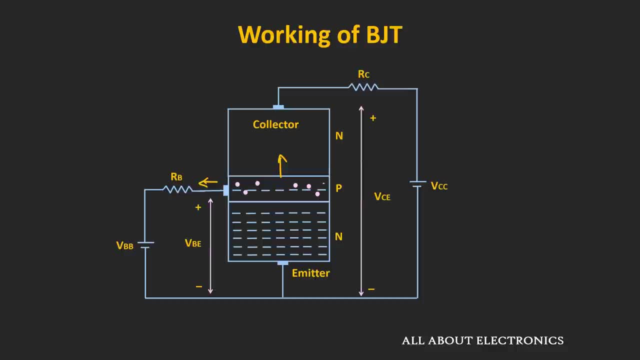 That means the number of holes in this base region is very small compared to the electrons which are coming from the emitter region. That means the free electrons which has come into this base region will see the longer lifetime. And the second reason is the width of this base region is very thin. 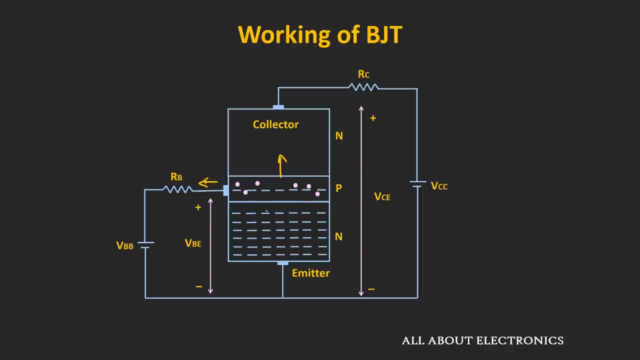 That means most of the electrons will be able to escape this base region And they can go into the collector region. That means in this base region only few electrons will recombine with these holes And they will get attracted towards the positive terminal of this VBB. 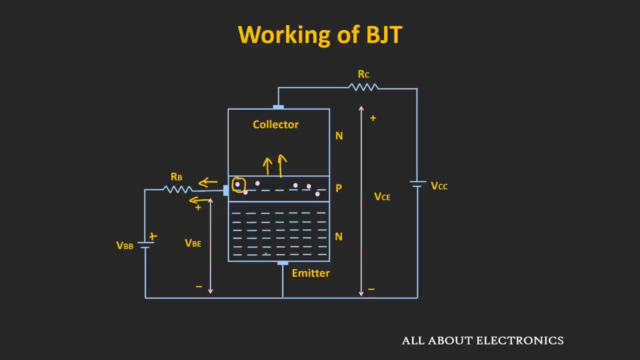 And the remaining electrons will enter into the collector region. Now, if you notice over here, once the electrons from the emitter enters into the base region, then they will become the minority charge carriers. And if you see over here, the base collector junction is reversed, biased. 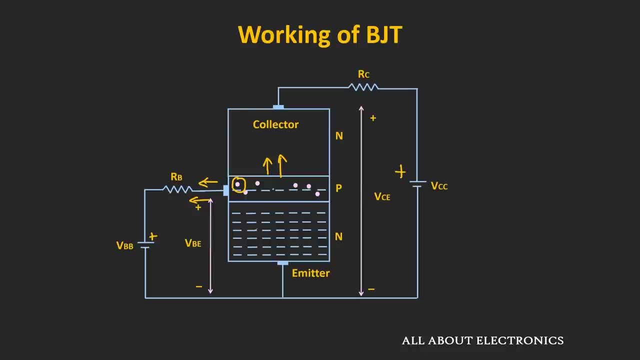 So, due to the applied electric field at the collector terminal, these minority charge carriers, or the electrons, will get attracted towards the collector terminal. So once the electrons enters into this collector region, then they will get attracted by the positive terminal of this VCC. 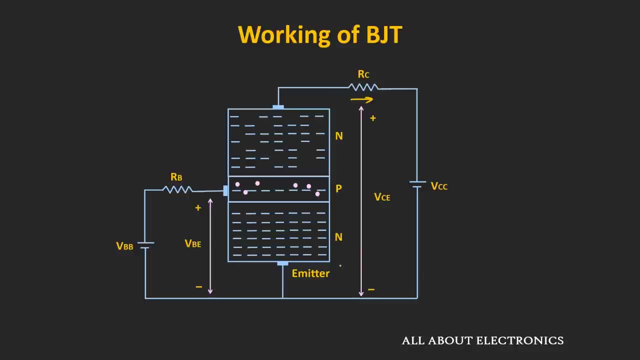 So if you see the direction of the flow of electron, then from the emitter the electrons will flow in this direction And most of the electrons which are emitted by the emitter will get attracted by the collector region And very small amount of electrons will get among the collector region. 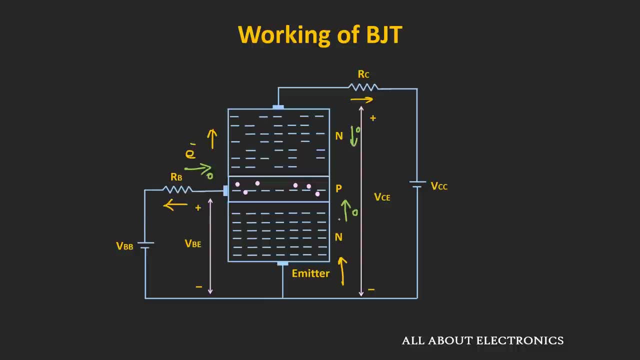 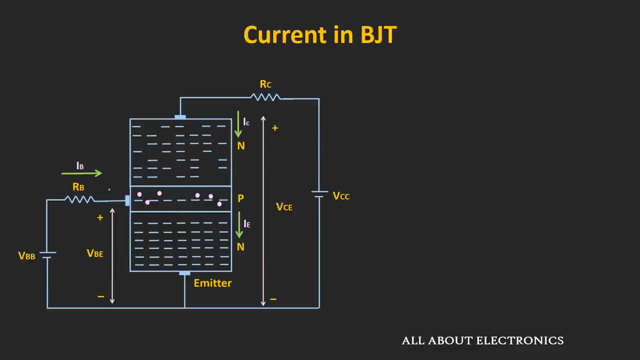 of electrons only will flow in this direction, And if we see the direction of the holes, then it will be exactly opposite to the flow of electrons And in fact the conventional current will also flow in the same direction. That means the base current Iv will flow in this direction. 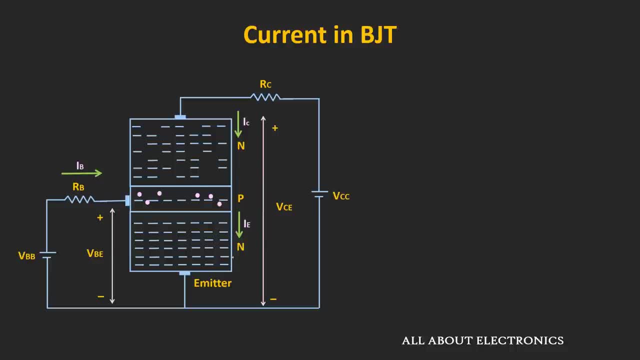 while the collector and the emitter current will flow in this direction. So now let's establish the relationship between all these currents. So if we apply the KCl, then we can say that this current Ib plus Ic, that is equal to emitter current. 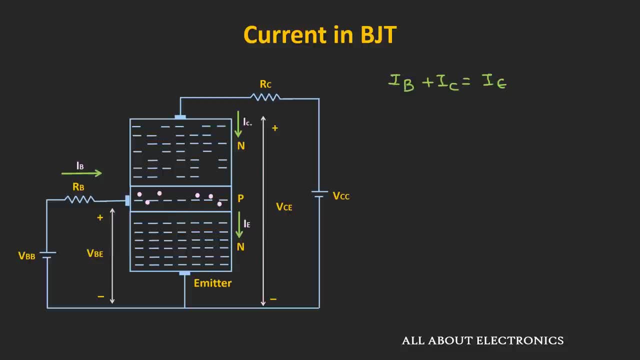 That means the emitter current is the summation of this base current and the collector current And, as I said, only fraction of electrons are able to go in this direction. That means the base current will be very small, Or we can say that this collector current Ic. 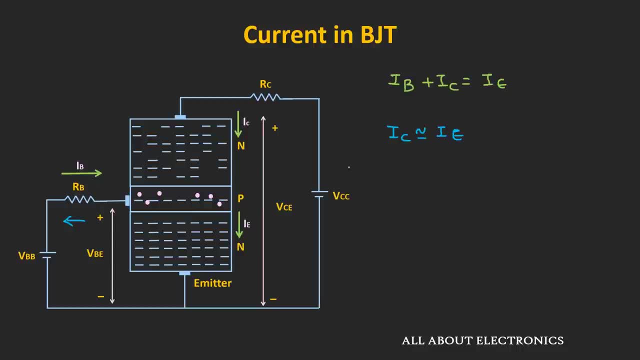 is approximately equal to Ie And exactly it can be defined as collector current. Ic is equal to alpha times Ie, And this alpha defines what fraction of the emitter current is flowing through the collector terminal. Now, if we put this value of Ic in this expression, 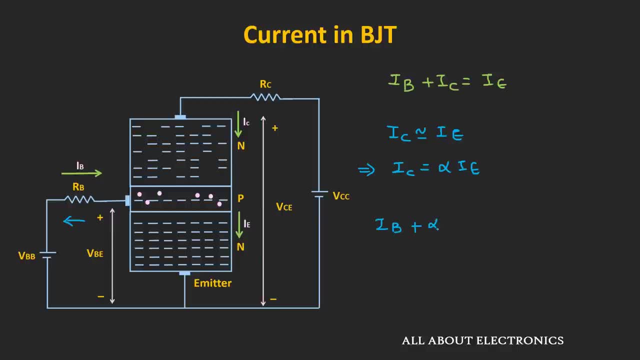 then we can say that this base current Ib plus alpha times Ie is equal to Ie. That means the base current Ib is equal to 1 minus alpha times emitter current. And once again, if we put the value of Ie plus alpha times Ie, that means the base current Ib is equal to 1 minus alpha times emitter current. 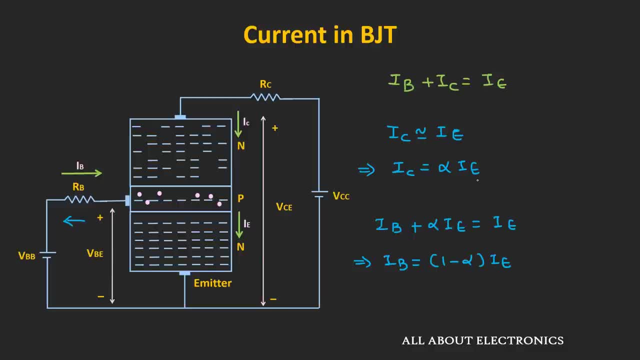 And once again, if we put the value of Ie in terms of the collector current, then we can say that the base current Ib is equal to 1 minus alpha times Ic divided by alpha. That means the base current Ib is equal to 1 minus alpha divided by alpha times collector. 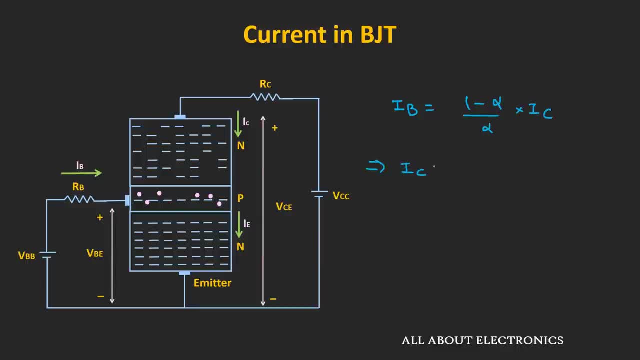 current. Or we can say that the collector current Ic is equal to alpha divided by 1 minus alpha times base current. And let's say that the collector current Ic is equal to alpha divided by 1 minus alpha times base current. Now let's write down the töaching equation to write down Ic as the collecting current of the cuma to thatants radio- 1996.. 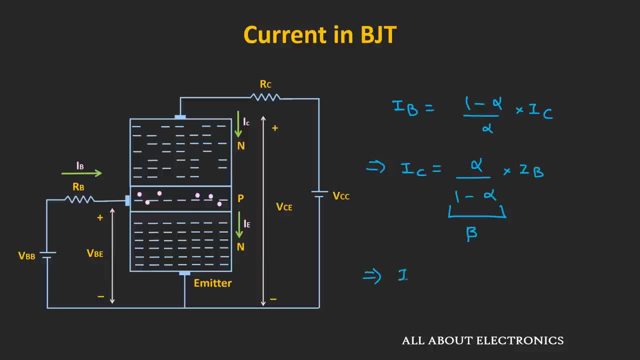 And let's say this is equal to beta. That means the collector current Ic is equal to beta times Ib. So this beta is known as the current gain of B, j, t, And typically the value of the β varies from 50 to 400 for the different transistors. So from thiswe can say that 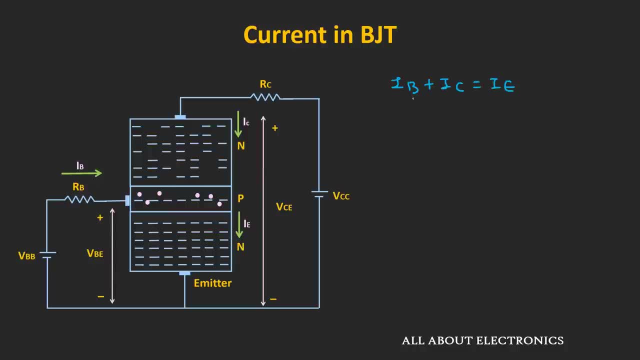 Ib plus Ic that is equal to emitter current. That means base current Ib plus beta times Ic is equal to Ib plus Ic. So that would indicate that the collector current Ic is equal to 1 minus alpha times beta, which means beta is one meter frequency down to one meter plus by other한 and five seconds. 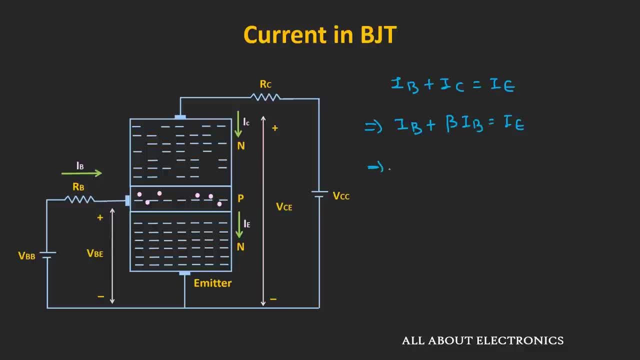 times Ib is equal to I. That means the emitter current I can be given as β plus 1 times Ib. So this is the relationship between the base current, emitter current and the collector current. Now if you notice over here, in this common emitter configuration this base current is: 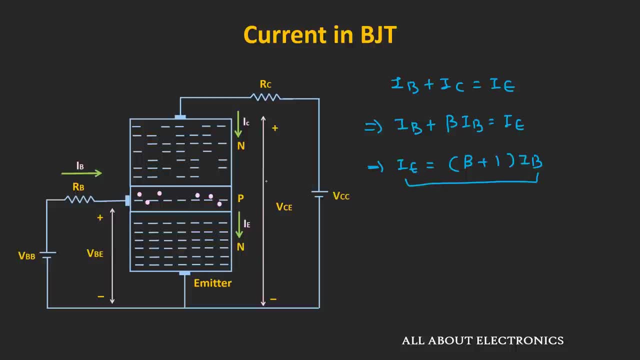 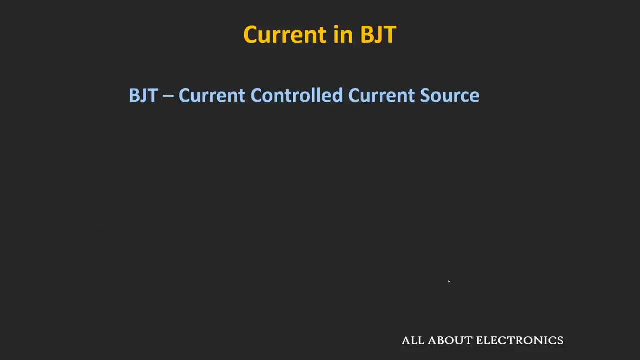 the current on the input side, while the collector current is the current on the output side And these two currents are related by this expression. That means by controlling this base current on the input side, it is possible to control the collector current, And that is why these bipolar junction transistors 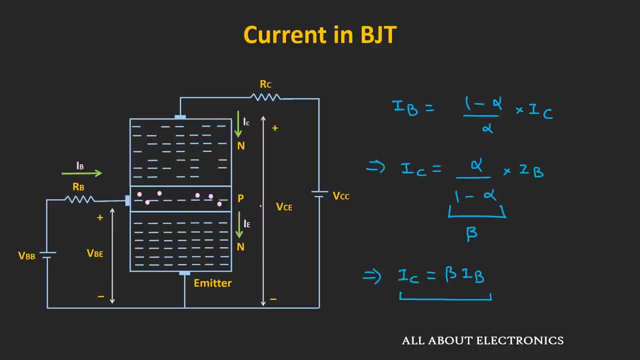 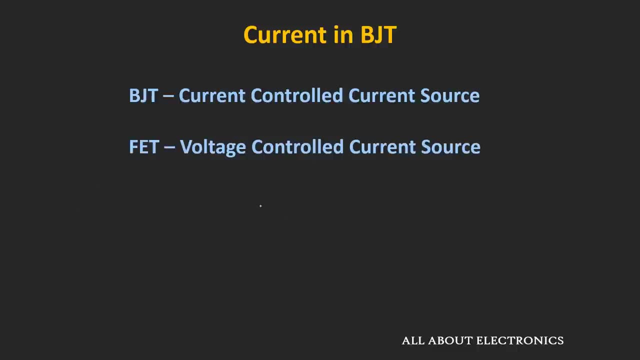 are known as the current control device. That means just by controlling the input current on the base side, it is possible to control the output current On the other end. if you see the other type of transistor, that is, the field effect transistor. 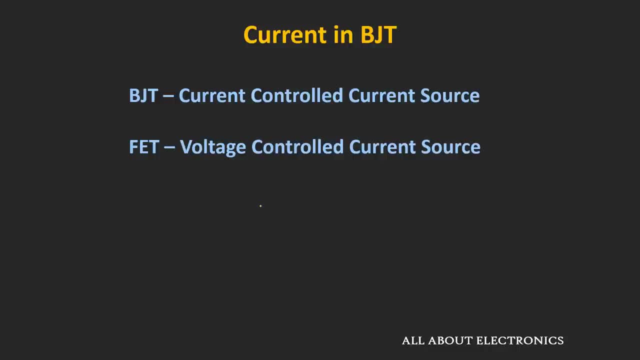 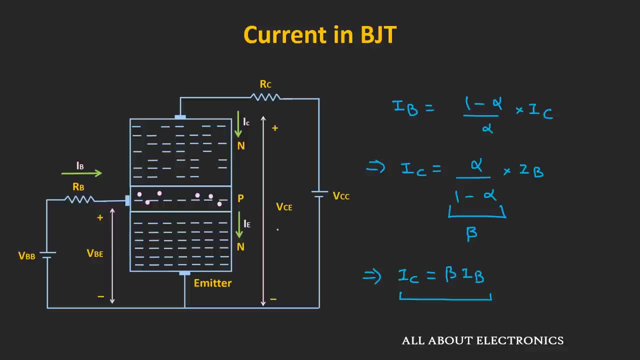 it is the voltage control device. That means in that case, by controlling the input voltage it is possible to control the output current. Also, if you notice over here, in this configuration of the BJT the output collector current gets amplified by the factor of β. 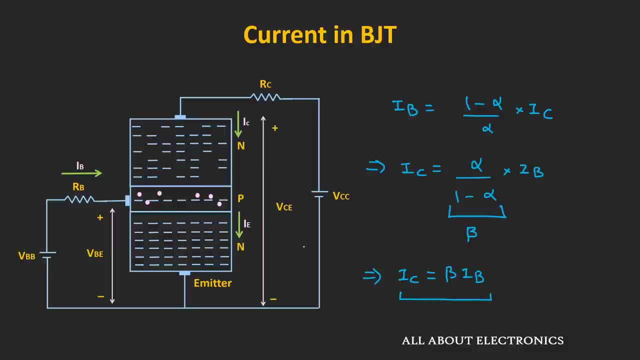 And if you connect the resistor between the collector and the emitter terminal, then it is possible to amplify the input signal. That means after biasing the BJT. in this configuration, if you apply the AC signal at the input, then it is possible to amplify that signal.